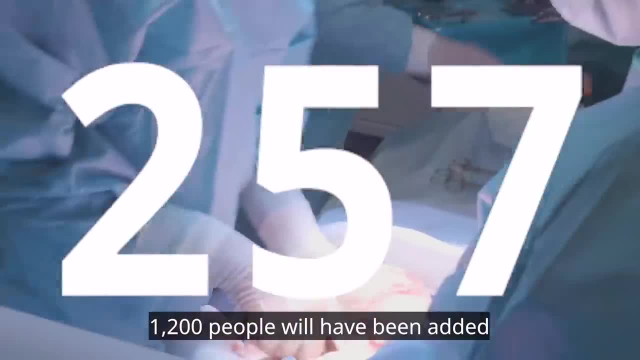 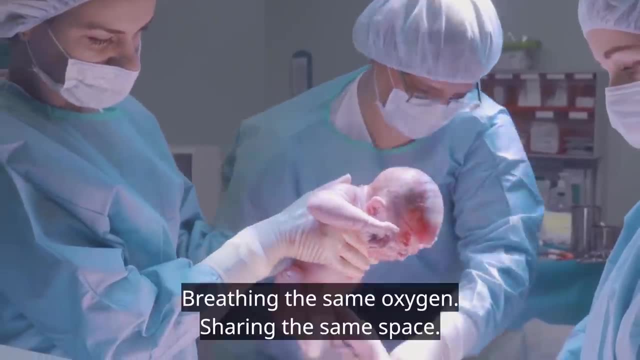 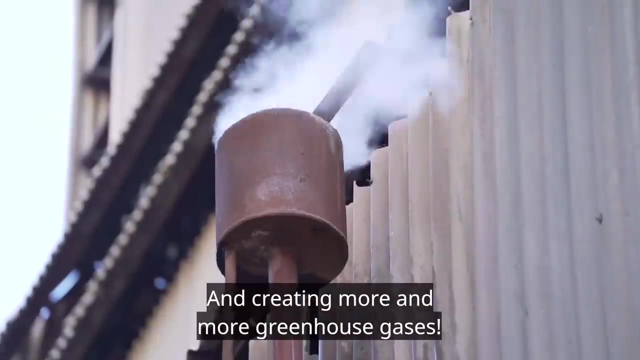 In the time you watch this, almost 1,200 people will have been added to our population, Breathing the same oxygen, sharing the same space and creating more and more greenhouse gases. Worries about overpopulation are back. We need to address much more aggressively. 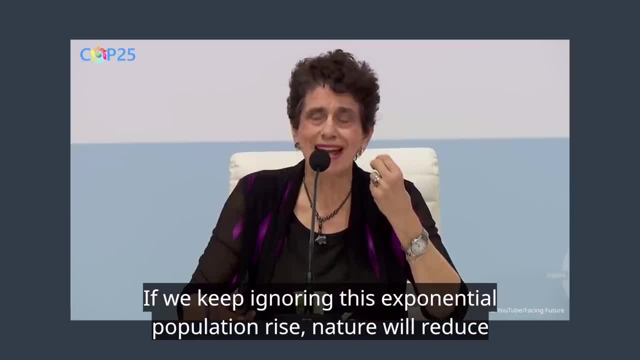 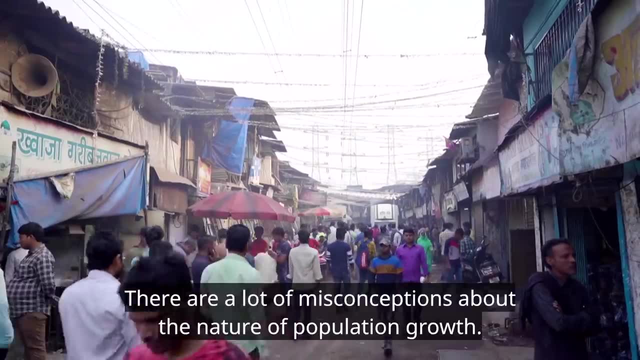 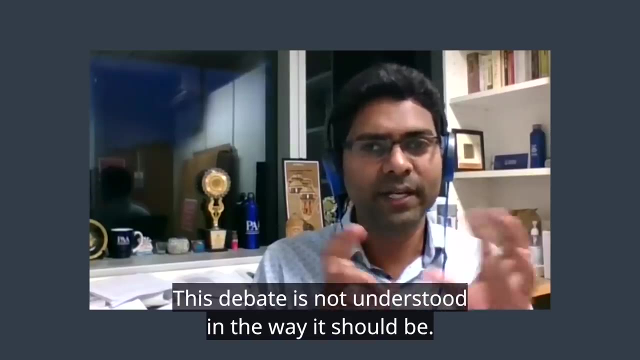 the population part of the equation. If we keep ignoring this exponential population rise, nature will reduce human population for us. Is this the whole story? There's a lot of misconceptions about the nature of population growth. This debate is not understood in a way. 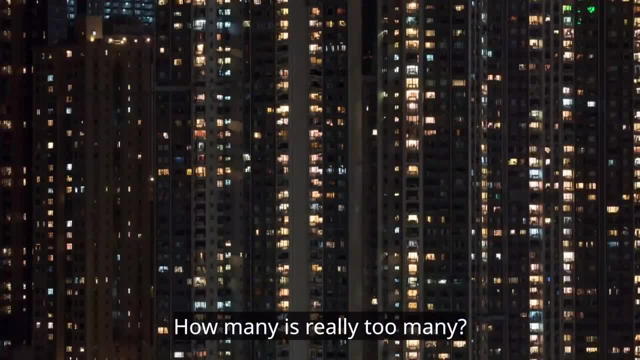 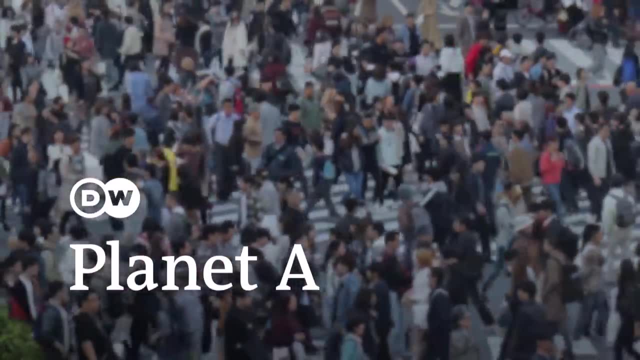 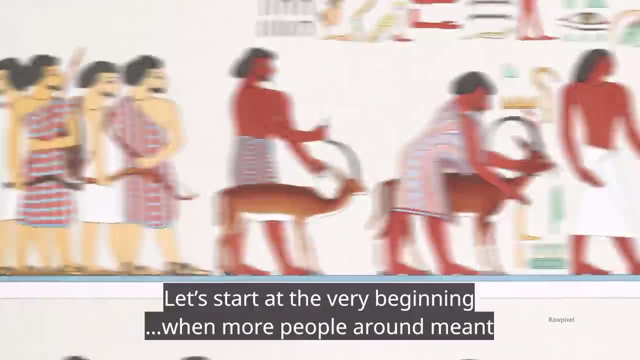 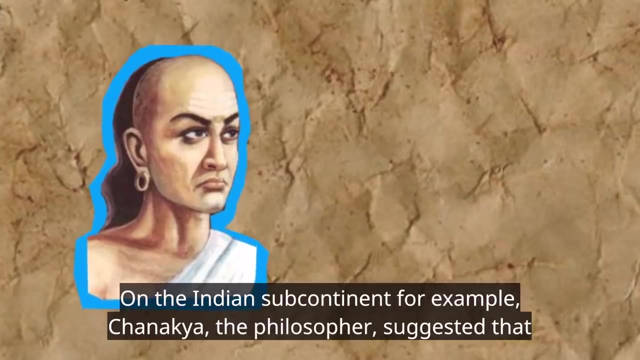 it should be. How many is really too many, And what does the answer have to do with frozen food? Let's start at the very beginning, when more people around meant security in an insecure world. On the Indian subcontinent, for example, Chanakya, the philosopher, suggested that widows quickly find 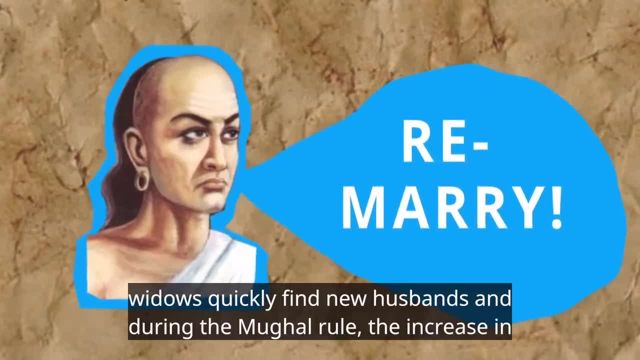 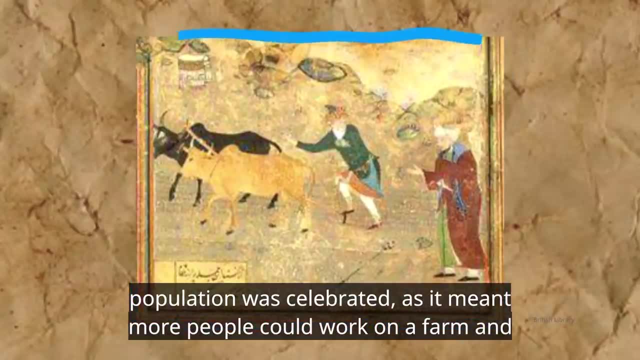 new husbands, And during the Mughal rule, the increase in population was celebrated, as it meant more people could work on a farm and produce more food. The Roman emperors were no different. They were the ones who made the most money. 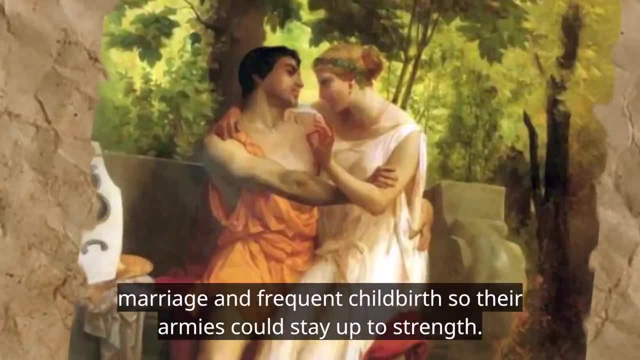 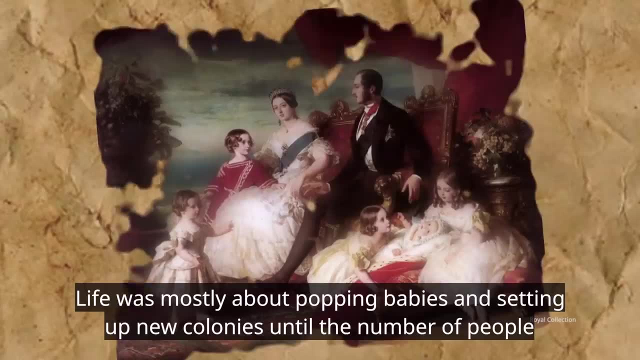 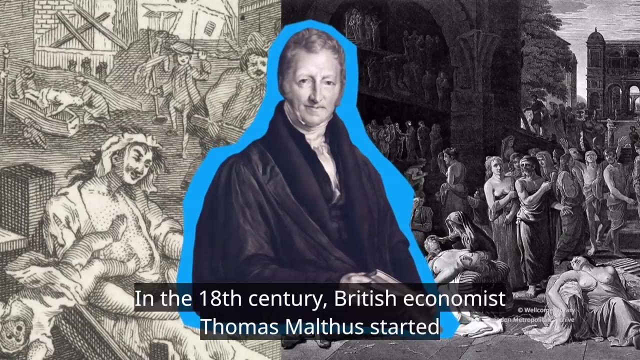 In some cases passing laws to promote early marriage and frequent childbirth so their armies could stay up to strength. Life was mostly about popping babies and setting up new colonies until the number of people started becoming a visible problem. In the 18th century, British economist Thomas Malthus started ringing alarm bells. 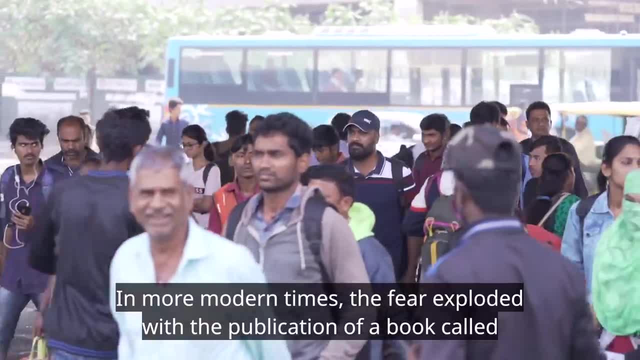 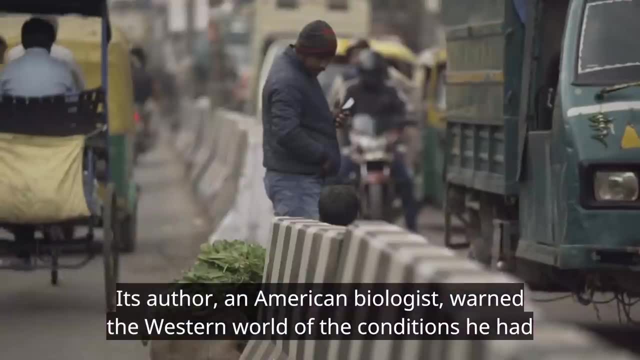 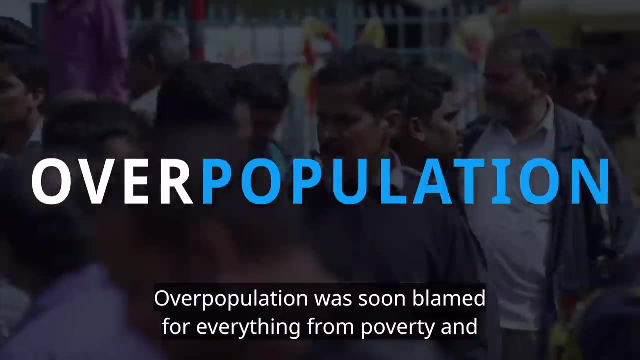 Okay, ancient history lesson done. In more modern times, the fear exploded with a publication of a book called the Population Bomb. Its author, an American biologist, warned the Western world of the conditions he had seen in New Delhi. Overpopulation was soon blamed for everything from poverty and poor resource management to destroying the environment. Some countries began experimenting with morally and politically dubious methods of population control. China became the poster child and its one child policy resulted in a disastrous gender imbalance And, like other control measures in Asia, it was eventually repealed. But the enemy had been identified as overpopulation. 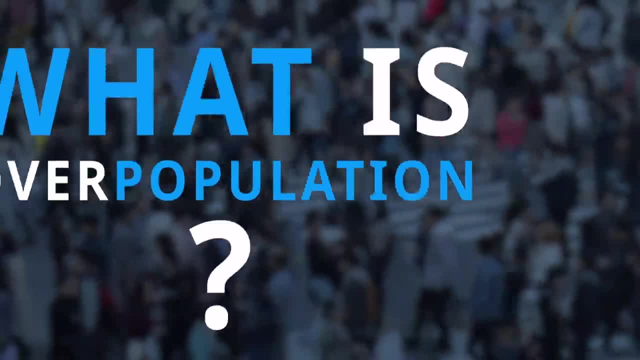 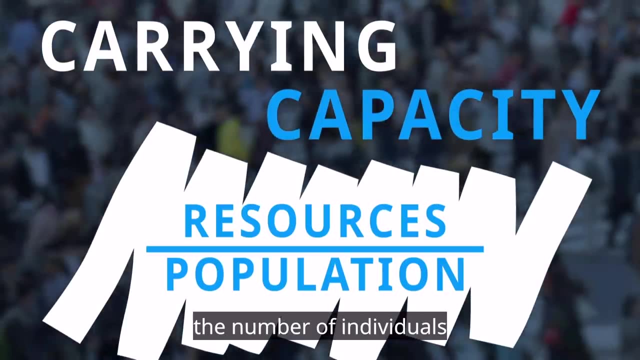 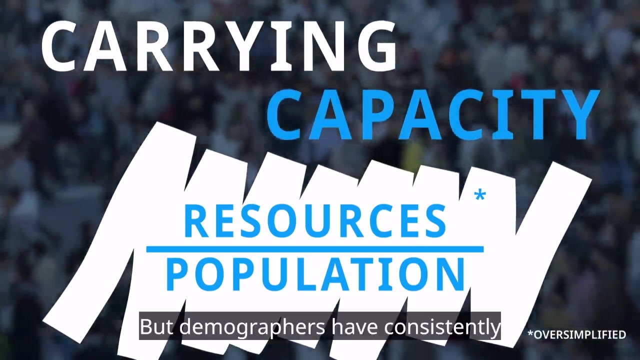 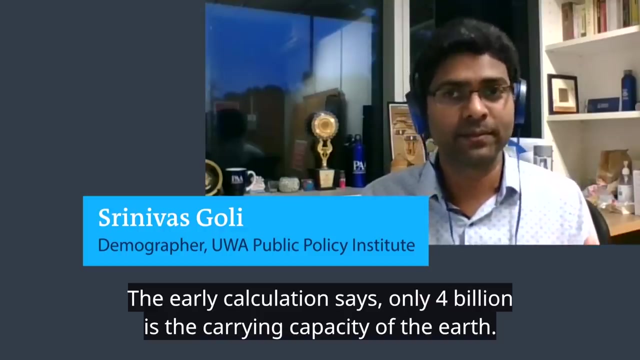 So what exactly is overpopulation? It is defined by carrying capacity, a slightly complicated concept, which basically means the number of individuals and ecosystems resources like food, water and space can sustain indefinitely. But demographers have consistently got it wrong. The early calculation says only 4 billion is the carrying capacity of Earth. 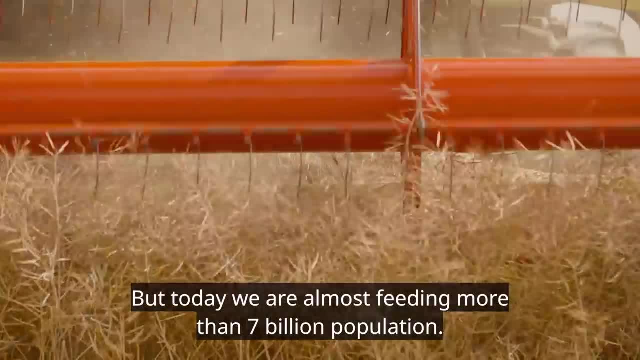 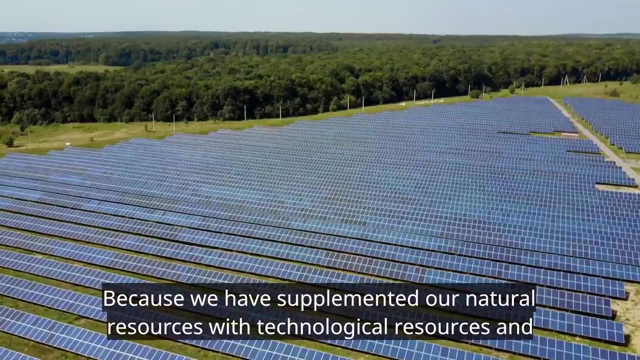 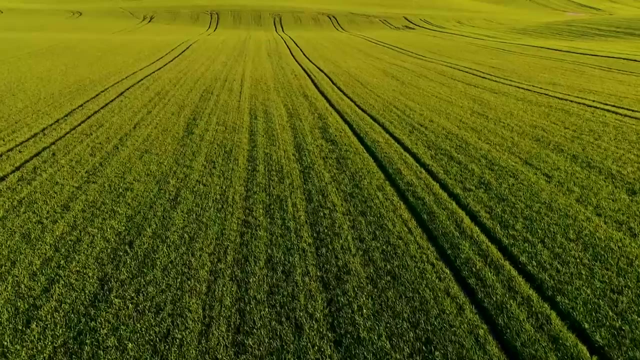 But today we are almost feeding the more than 7 billion population because we have supplemented our natural resources with the technological resources and we have to use the resources to sustain the population. So we're not quite sure what the Earth's carrying capacity is, because the variables are. 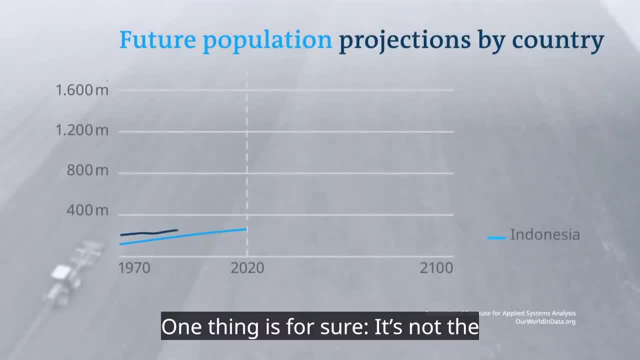 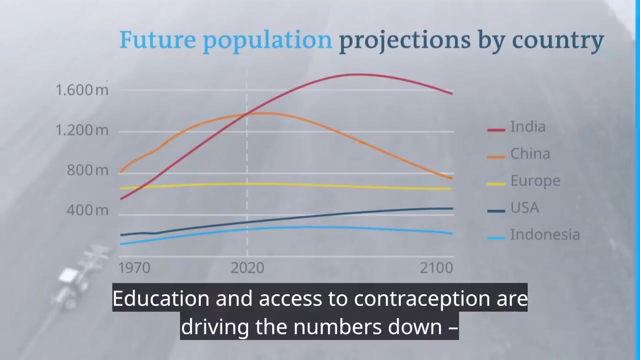 constantly changing. One thing's for sure: it's not the population element that's going to be the problem. Already in the developed world, the population has largely stabilized or begun to decline, And the developing world is on track to follow. Education and access to contraception. 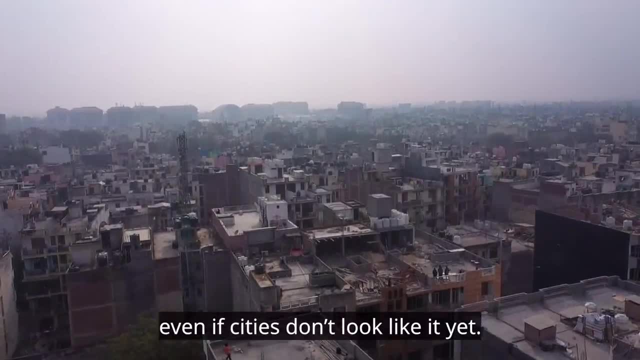 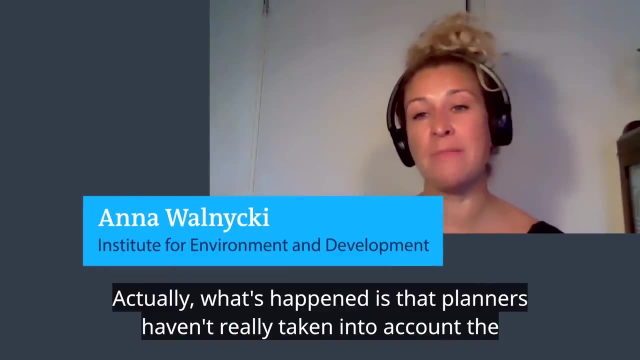 are driving the numbers down, even if cities don't look like it. yet People get this perception that these cities are overcrowded and they're really busy. Well, actually, I think what's happened is that planners haven't really taken into account the population growth. 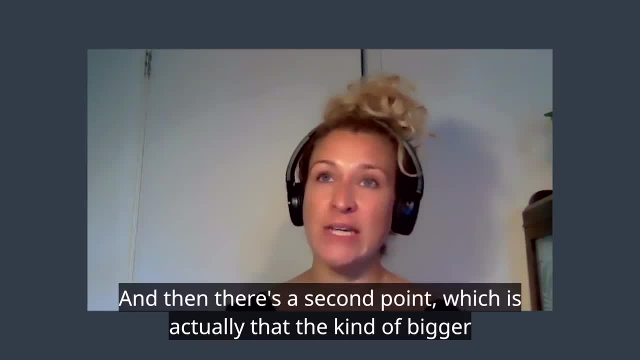 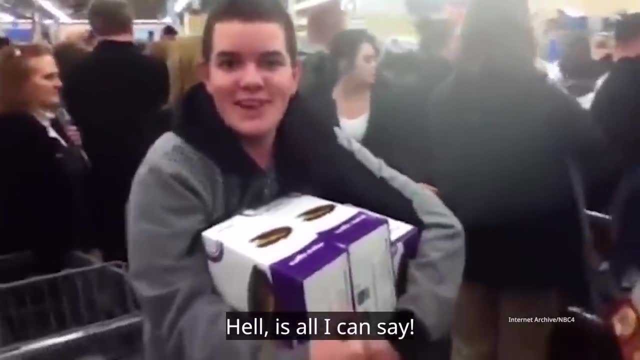 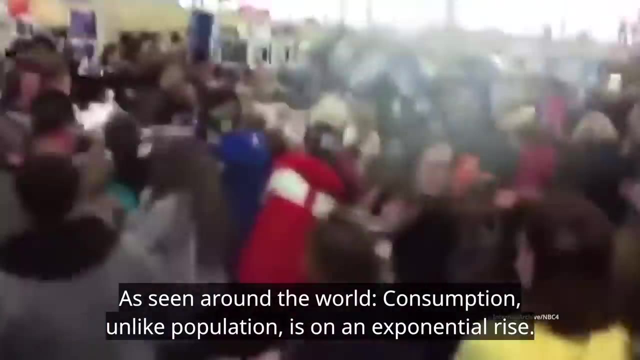 that's going to happen anyway. And then there's a second point, which is actually the kind of the bigger impacts on the environment are linked to consumption. As seen around the world, consumption- unlike population- is on an exponential rise. If we look at our levels of consumption across different contexts, 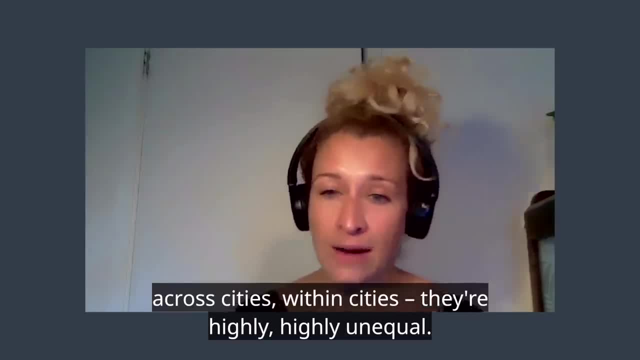 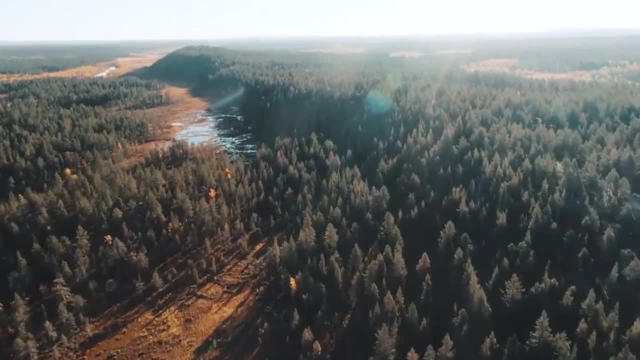 globally, across cities, within cities, they're highly, highly unequal. OK, so let's then look at how we are consuming resources in that equation. Every year, researchers look at the Earth's annual resource budget and calculate at what point we will use it up. 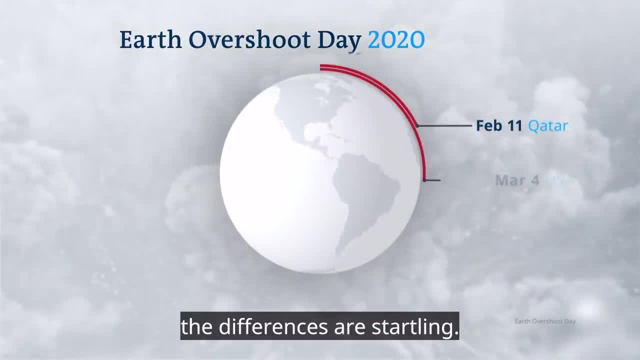 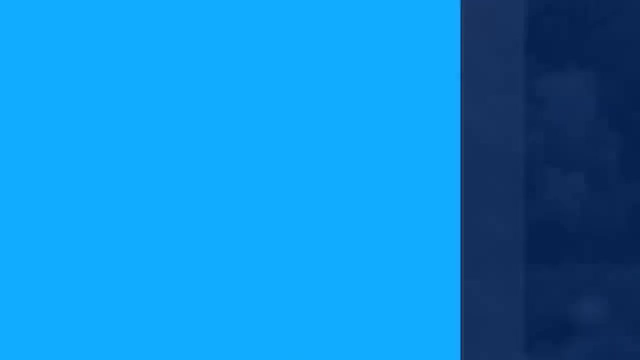 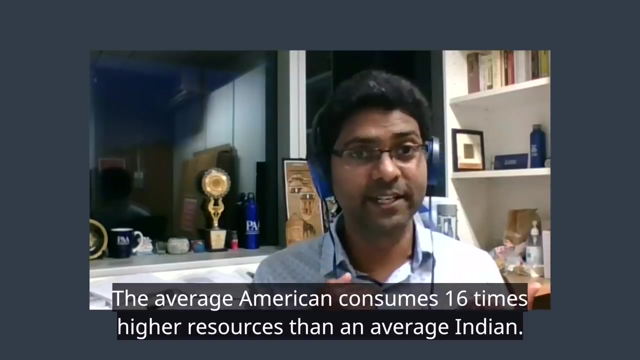 If we look at this by country, the differences are startling. Many nations in the Middle East and West exhaust that budget in the first quarter, while a few countries like India don't. And they don't overshoot yet. The average American consumes 16 times of higher resources than an average Indian. 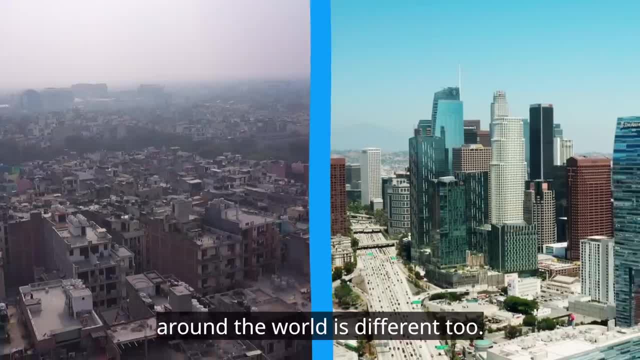 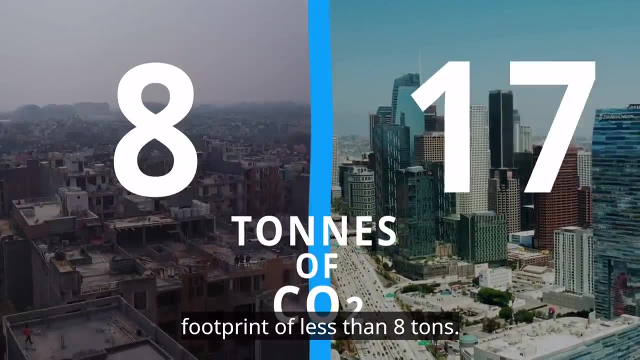 And, correspondingly, how much carbon dioxide we emit around the world is different too. In 2018,, an Indian family of four had a carbon footprint of less than eight tons. An American family of four in the same year had a carbon footprint of less than eight tons. 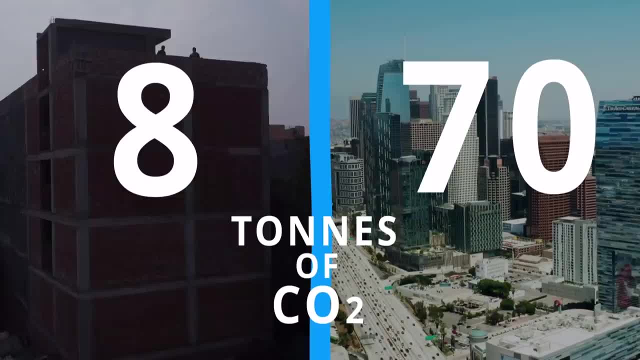 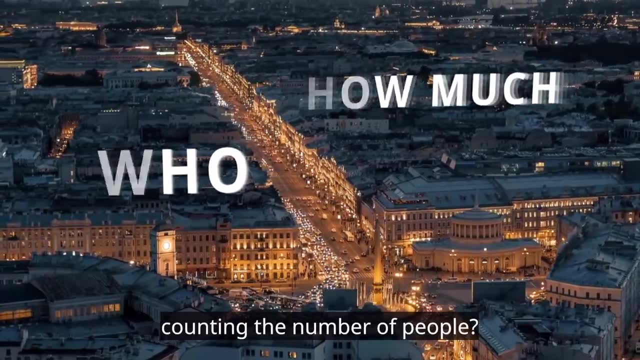 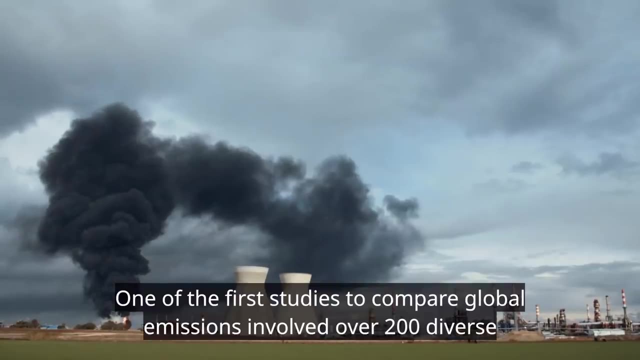 And in 2018, an Indian family of four in the same year came in at almost 70.. So shouldn't we then be looking at who is consuming and how much, instead of simply counting the number of people? One of the first studies to compare global emissions involved. 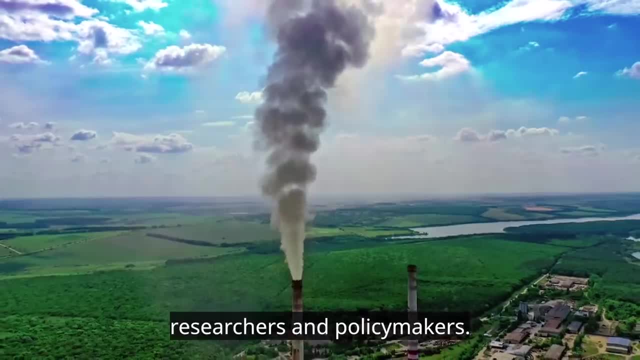 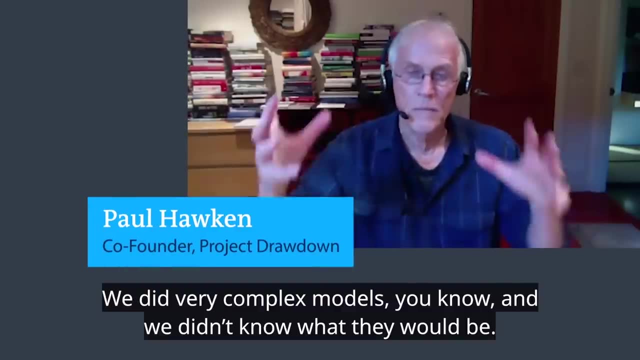 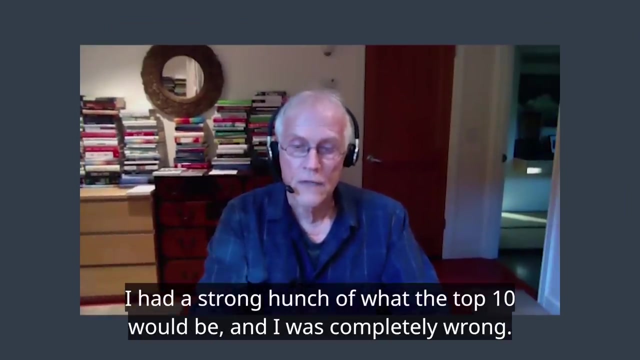 over 200 diverse researchers and policy makers. The result, called Project Drawdown, published a definitive list on reducing our impact. We did very complex models, you know, and we didn't know what they would be. I had a strong hunch of what the top 10 would be. 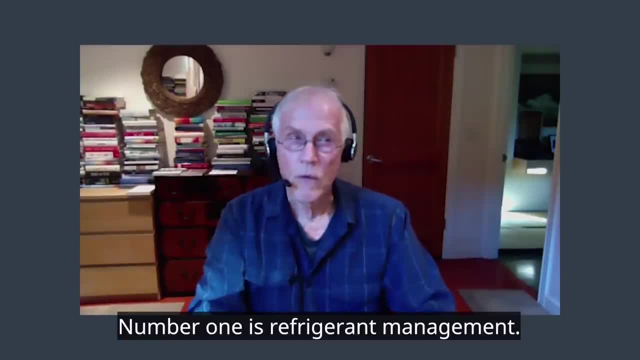 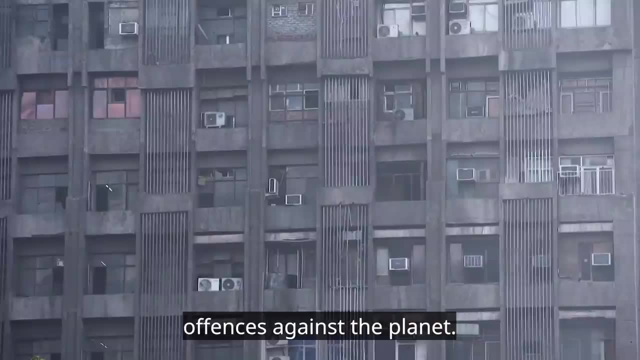 and I was completely wrong, and all the rest of us were wrong. Number one was refrigerant management. Yes, you heard that right. The way we keep things cool is one of our worst offences against the planet. Our air conditioners and refrigerators still largely emit greenhouse gases. 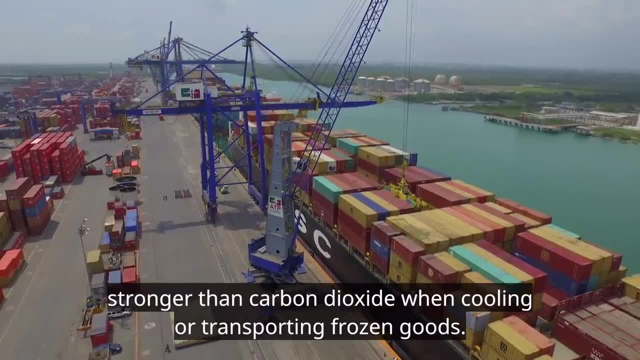 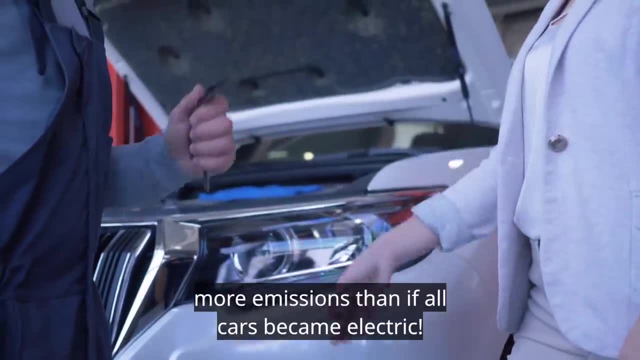 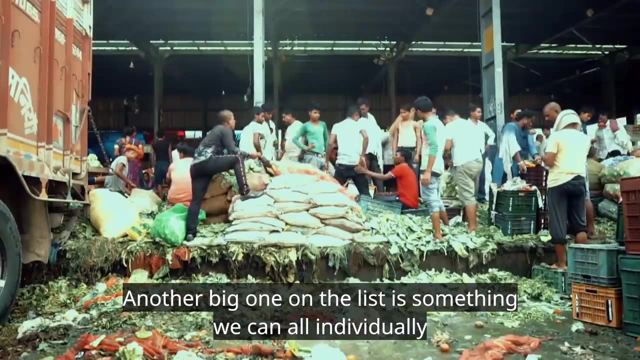 much stronger than carbon dioxide when cooling or transporting frozen goods. The project estimates that changing to more efficient cooling could save five times more emissions than if all cars became electric. Another big one on the list is something we can all individually do something about: Food is huge. 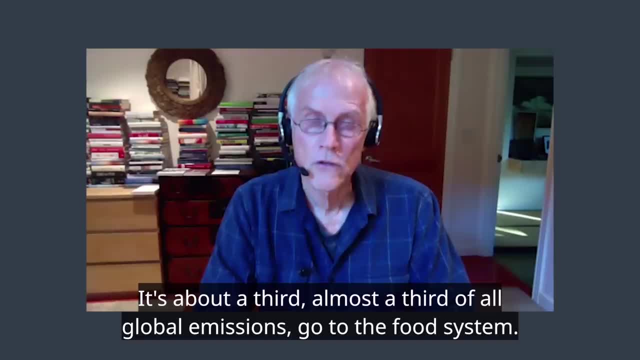 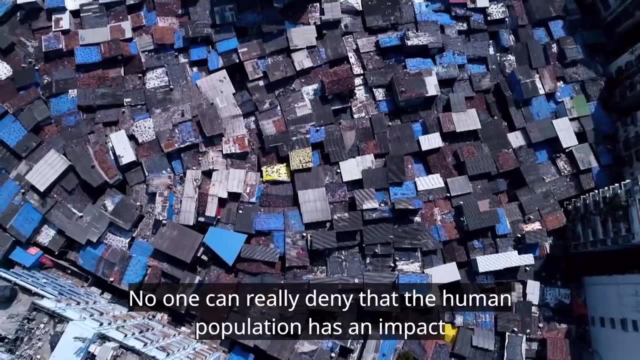 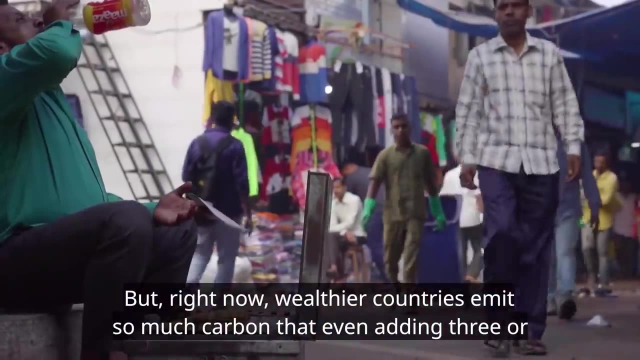 It's about a third. almost a third of all global emissions go to the food system. Waste nothing, if possible. No one can really deny that the human population has an impact on the environment, But right now wealthier countries emit so much carbon. 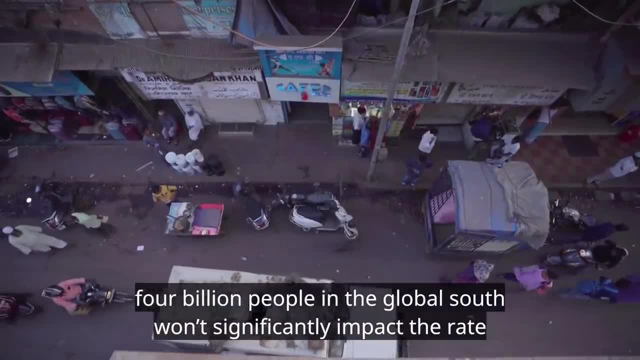 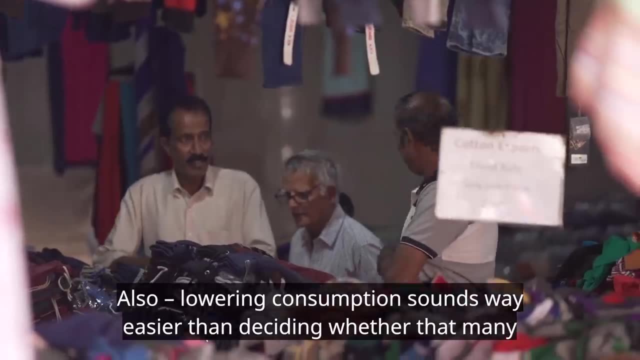 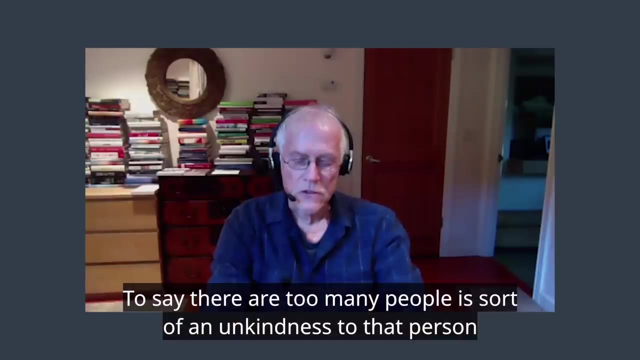 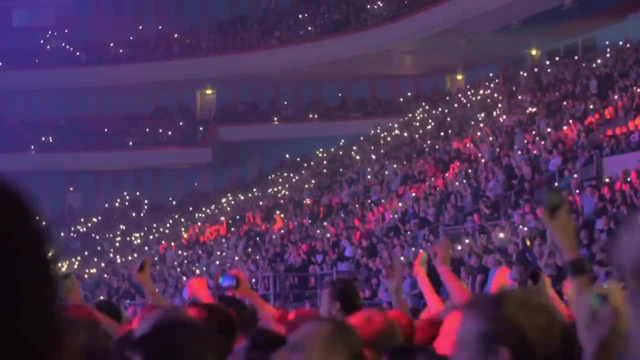 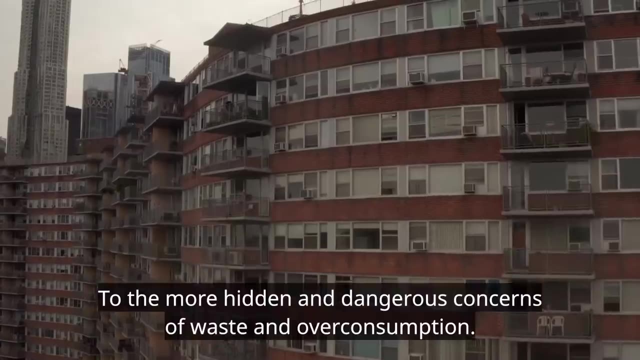 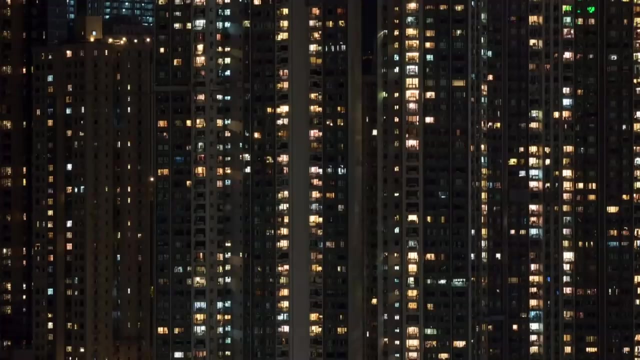 Like the person thinks there are too many. No one. It's time to change the narrative away from the easy-to-blame visual problem of population to the more hidden and dangerous concerns of waste and overconsumption. We try to answer the biggest questions concerning climate change today. 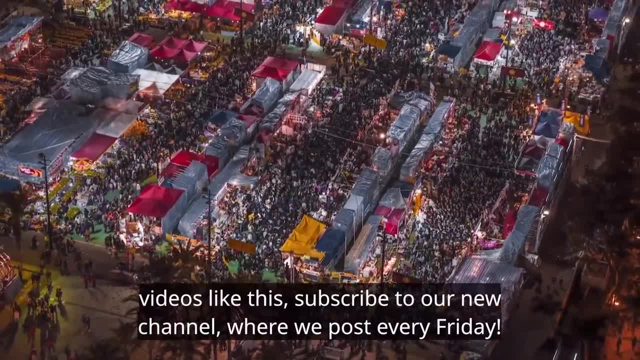 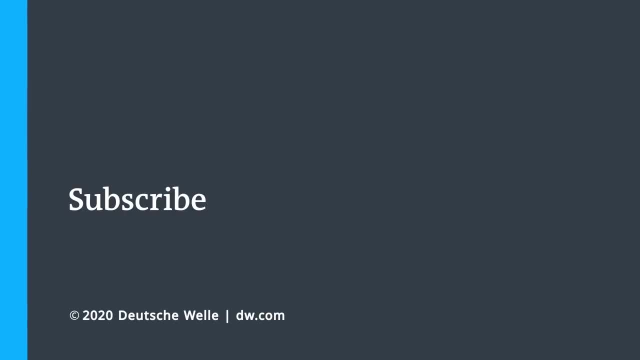 For more videos like this, subscribe to our new channel, where we post every Friday. Thank you. 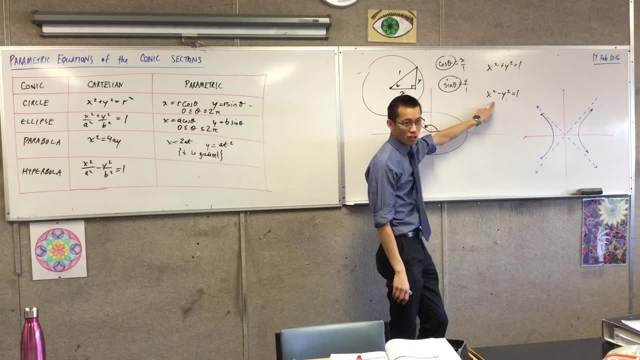 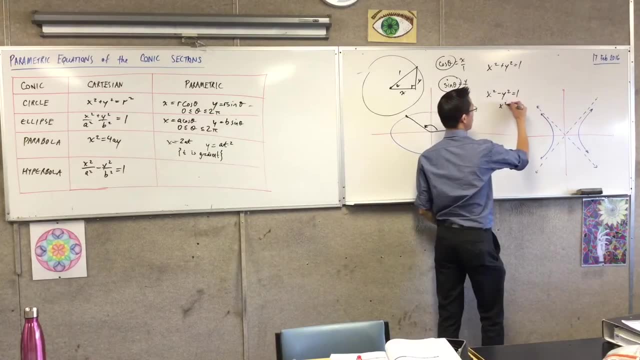 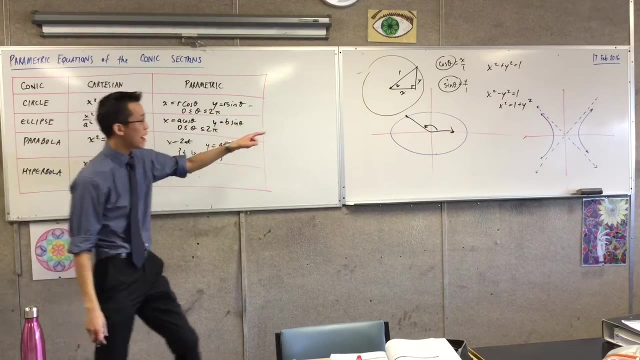 This is not a right angle triangle, At least not in its current form. I have a difference here, not a sum. In order to make it clear what's going on here. I just need to adjust it ever so slightly. Now I have a right angle triangle, I can form a right angle triangle kind of like this one. 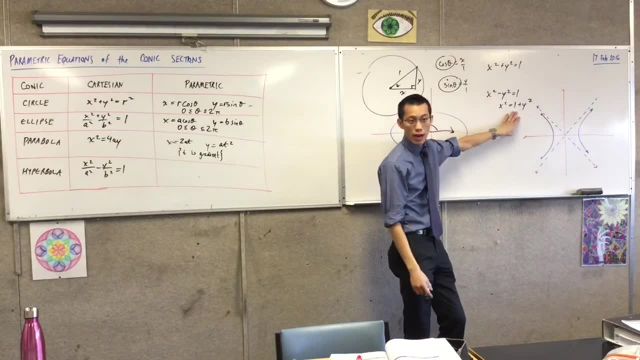 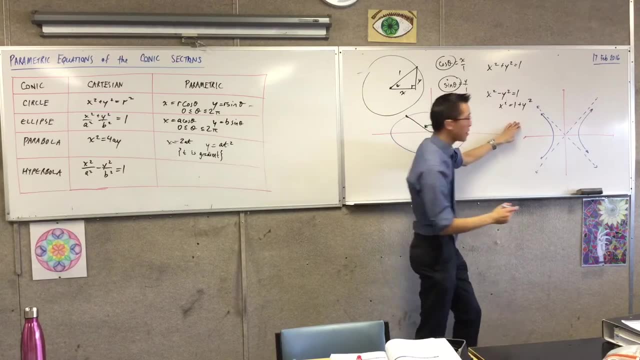 It won't be like this because I'm not in a circle anymore, But I can form a right angle triangle where the sides behave like this. They give me this Pythagorean theorem in this particular arrangement, So draw with me a right angle triangle. 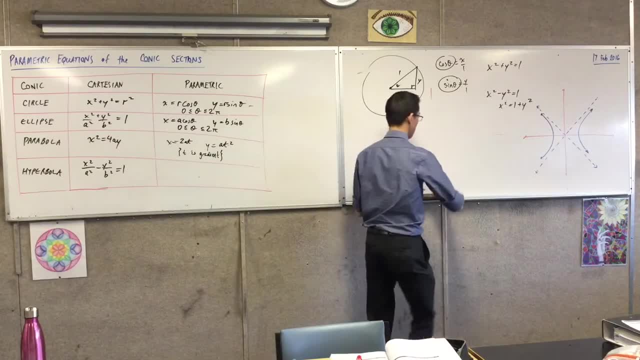 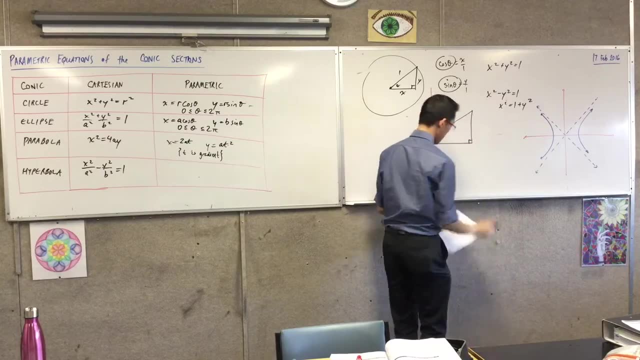 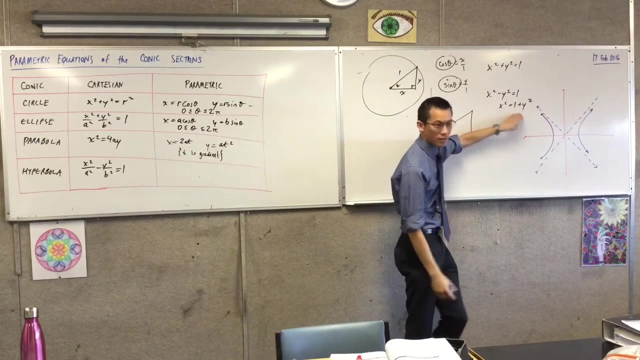 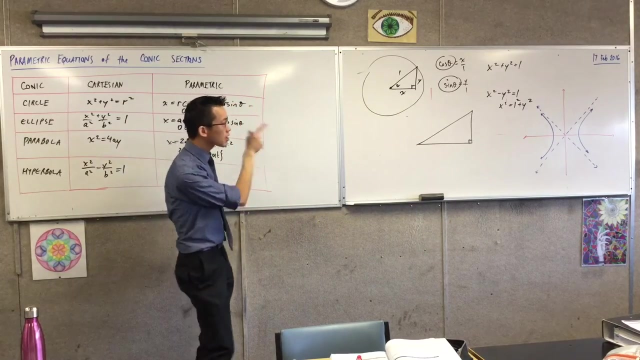 Just a simple one like this one Now, because I've got x squared on the left and then I've got 1 squared and y squared on the right. What that means is, in our fictional right angle triangle, x squared or x is which side. 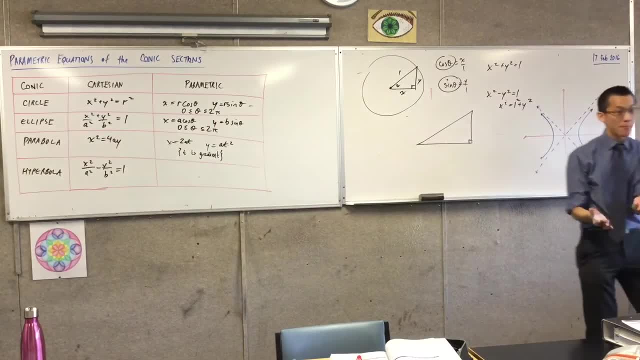 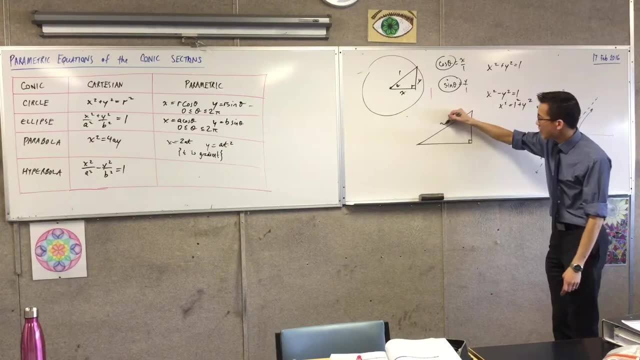 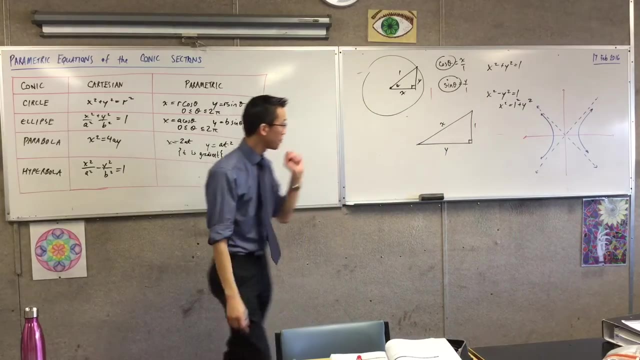 Which side is it? According to Pythagoreans, It's the hypotenuse, is it not? It's the biggest side, And these two are the squares of the smaller sides. So that means x is over here, And then, in some arbitrary sense, that means I'm going to have a 1 and a y on the other two sides. 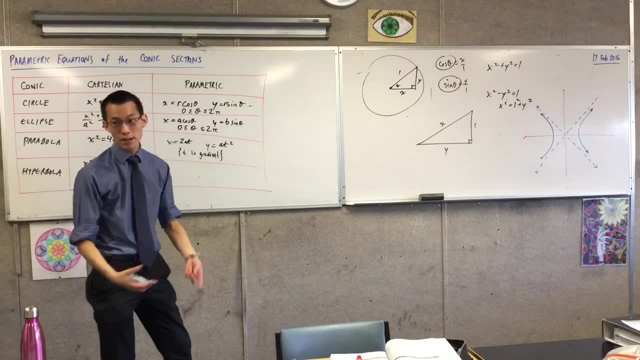 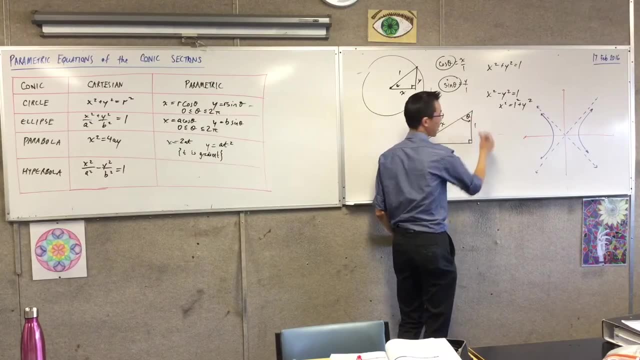 Now our next step is a bit arbitrary, But we've done this as mathematicians, just so we have a bit of consistency And the maths does end up being slightly simpler. If I put theta up here, I really could put theta in either spot.